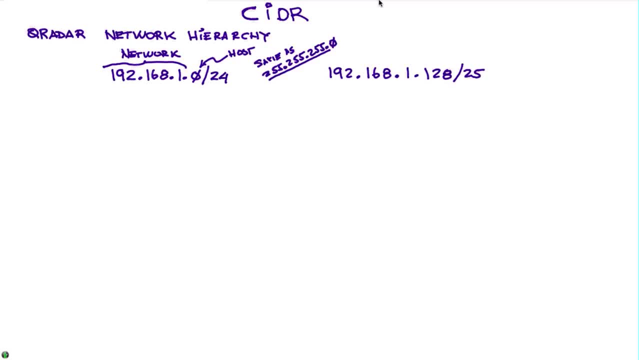 but 128 slash 25. what does that mean? well, these are two subnets, and, and the way that you, an easy way that at least I use for remembering this is: you know, the IPv4 is a 32-bit address space, so what you do is that you. 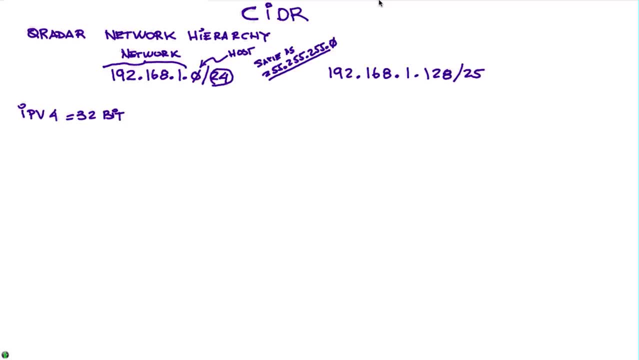 take the stuff after the slash and you subtract it from 32, so 32 minus 24, that's 8, and 2 to the 8 is 256. in this particular case, 32 minus 25 is 7,, so 2 to the 7. 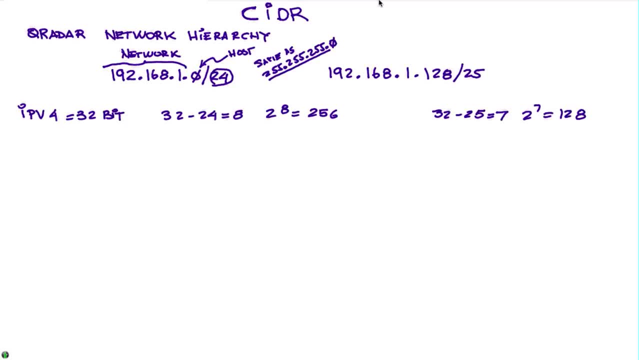 this represents 128 addresses on that particular subnet. so as you increase this stuff that comes after the slash, the smaller the network becomes. so this address, let's go back to the 192.1, 168.1, slash 24. that represents a network address that goes from 192.168.1.1. 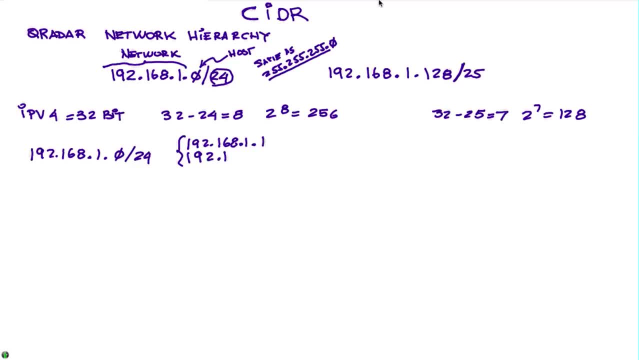 through 192.168.1.254. why is that? well, the .0 always is the name of the network specifying the subnet, and the .255 is the broadcast. so you cannot assign any one of those to network, and every time you divide a subnet. you cannot lose those two addresses because for that subnet the first represents the network. so for example, I can. this address on 25 is an address that goes from 192.168.1.129, again one more until 192.168.1.129. 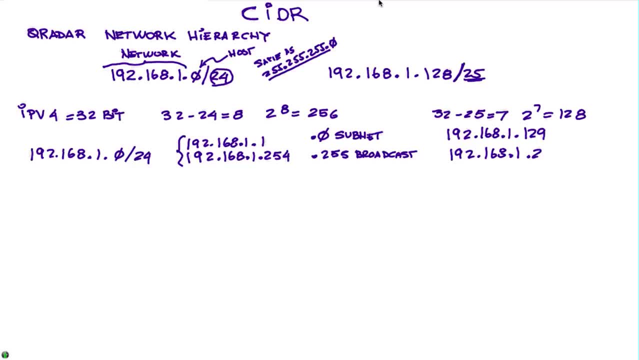 .1.129, again one more until 192.168.1.129. .1.129, again one more until 192.168.1.129 .1.254. so again, in this particular case, we have divided this 24 subnet with 256. 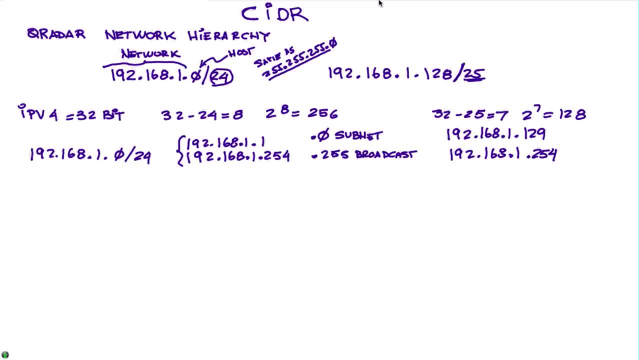 elements into a subnet that has 128 each, as you can see here. let me give you some some other example. so let's say that we want to subdivide this further. we had 192.168.1.128- .1.128.24 and we want to divide that by 2.